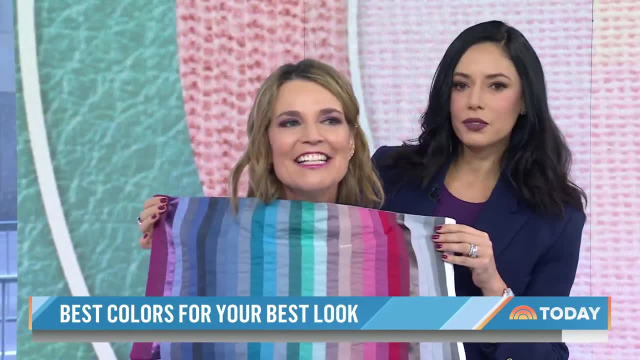 This is better. Yeah, It connects to you. It's brightening your face. Yes, it's brightening your face. Okay, Very cohesive, Okay, So that's the color Summer. I'm a summer, You're a summer. 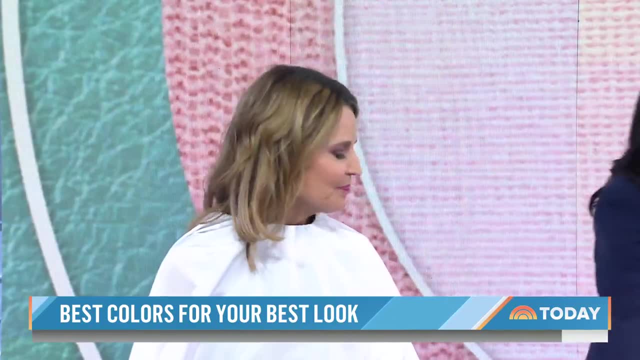 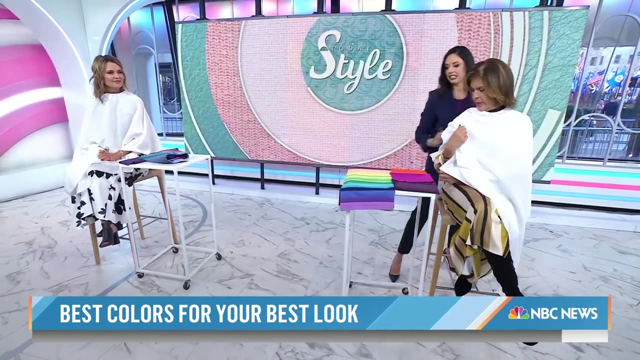 Yes, Oh, I was shocked. I would have thought it was a winter. Okay, How about Hoda? Okay, Hoda, let's do it. Okay, Take this out. And Hoda has a warm undertone. Take this out, so it doesn't Okay. And let's um, um, let's try some palettes. So we're trying. 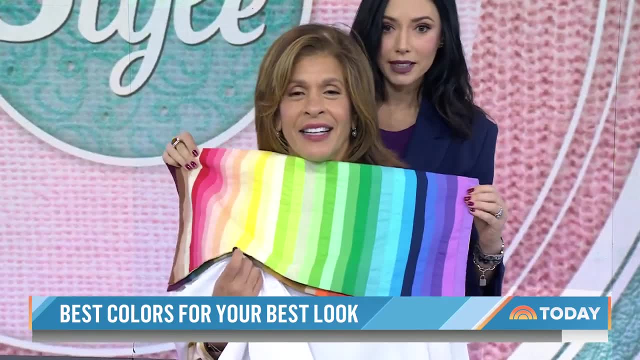 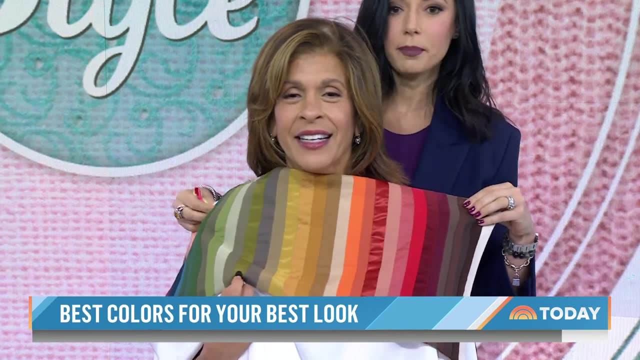 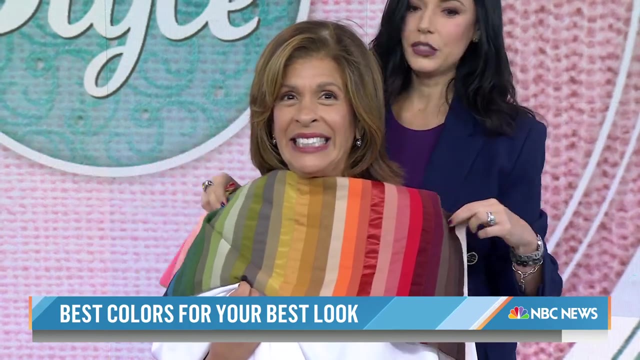 spring, which is very light and bright palette versus- I like that, I like that, You know- likey Spring versus autumn, which is more deep and muted. What do you think? Probably autumn blends better, but I kind of like the bright poppy. I understand, but where's the brighter? 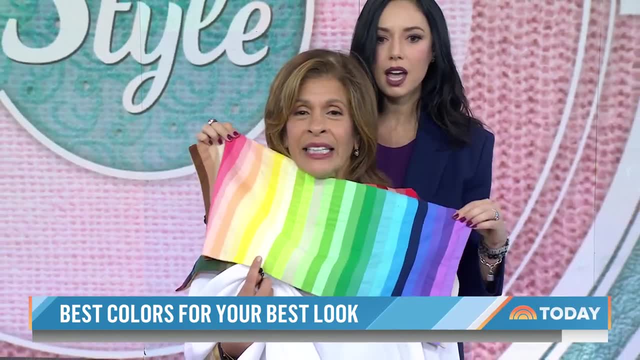 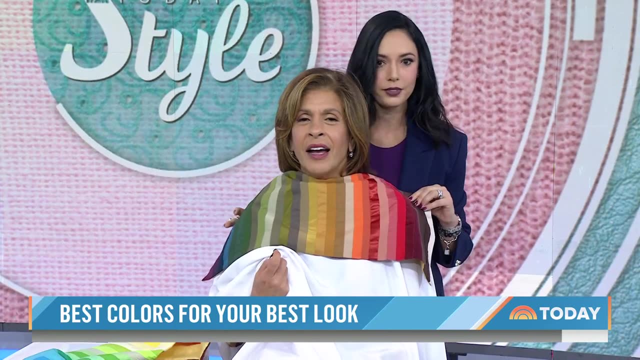 colors. What happens is your face becomes more pale, Oh yeah- And washed out. Not good, Not good, Julia. And it doesn't connect to you. It's really overpowers your look because it steals the attention from your beautiful face. So Someone repeated that loudly. I. 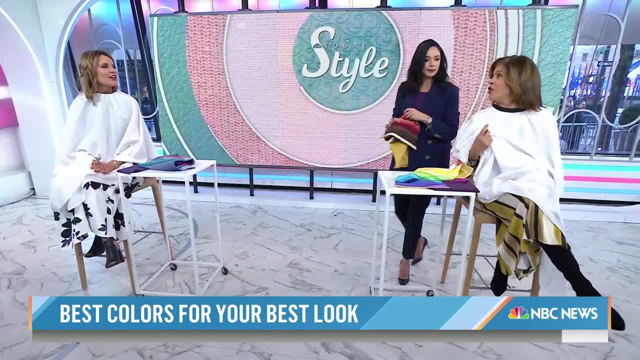 think this one, This is the one. So I'm a- what am I again? Autumn. I'm a fall, Winter, You're an autumn. You're a summer, Summer, I'm shocked Okay, Autumn. So what do people? 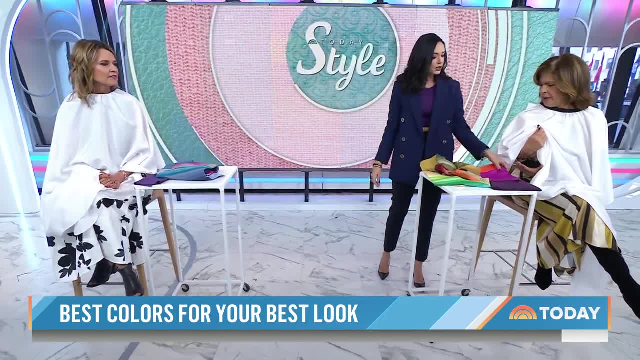 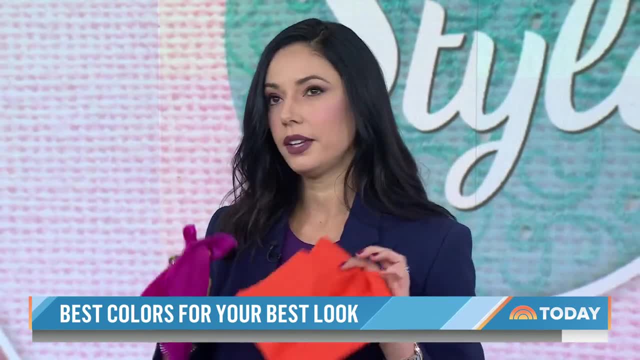 at home who are watching, going like I want to know my palette. How do you even begin to figure it out? I think to begin you have to do the undertone first and you've got to know what colors are cool, what's warm. So I think the face that the very safe choice. 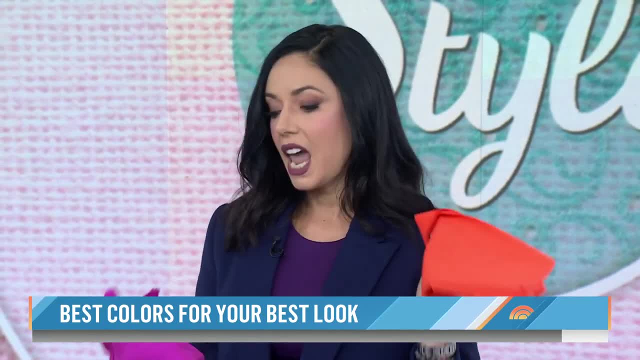 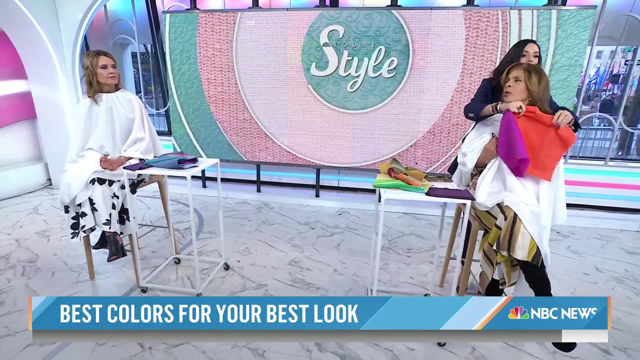 is to go with um a magenta, which is always cool, Yeah, And um and um, which is always warm. So I will show you, I look terrible in green. You think, Yeah, Okay, That's an. 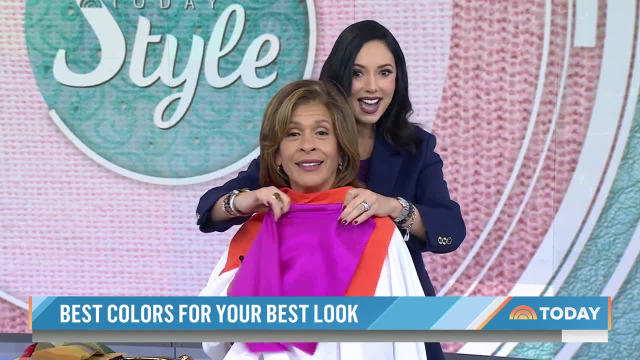 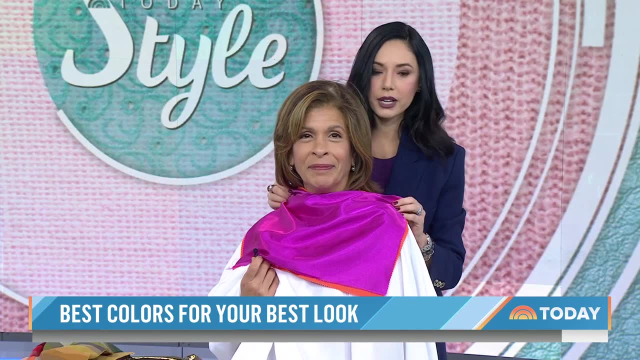 awesome. This is an awesome color. This is an awesome color. I can wear this. Yeah, And this and this one is the. you have that cute jumpsuit in that color. It makes you overpowering for you. It creates a lot of grayness on your face. Yeah, And look at this When we do this. 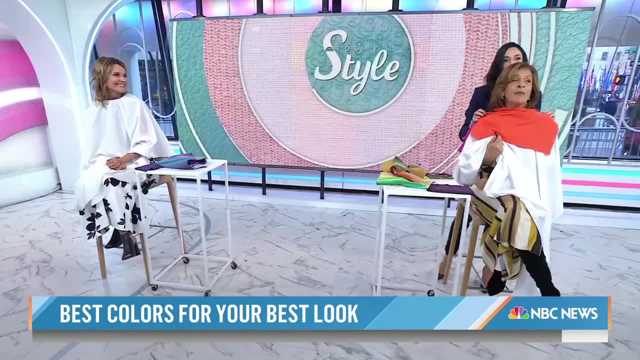 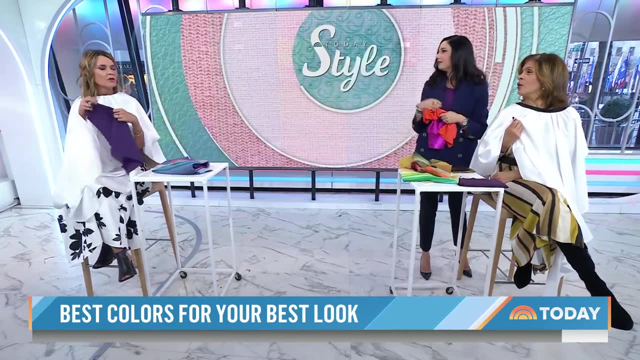 your face brightens up, right, Okay, You are glowing. I think I'm going to get orange. We got to go. Yeah, We're out of time, So okay. So now we know, Yes, we do Warm Cool.